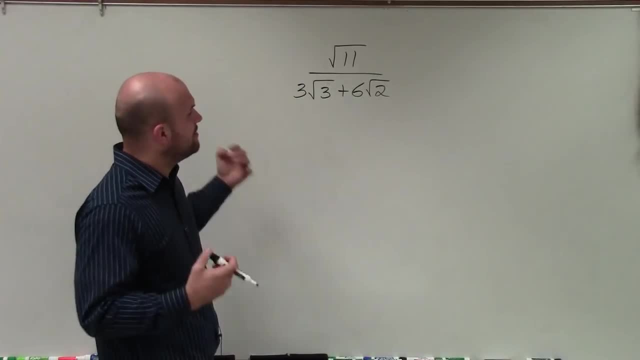 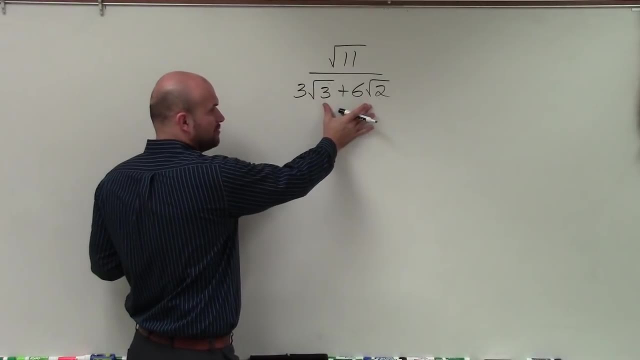 the denominator with a binomial. as your denominator, we want to be able to multiply by the conjugate. So to multiply by the conjugate. basically, what we're going to have is the exact same binomial, But rather than being separated by addition, we're going to separate by subtraction. 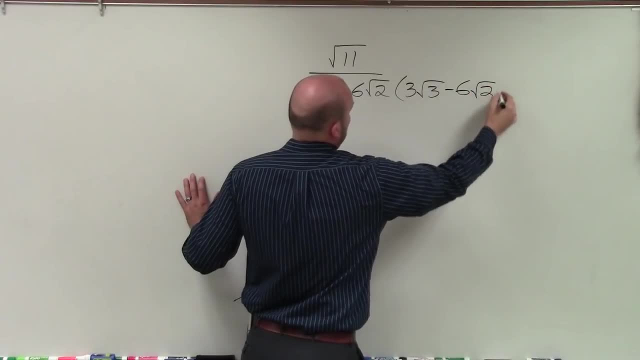 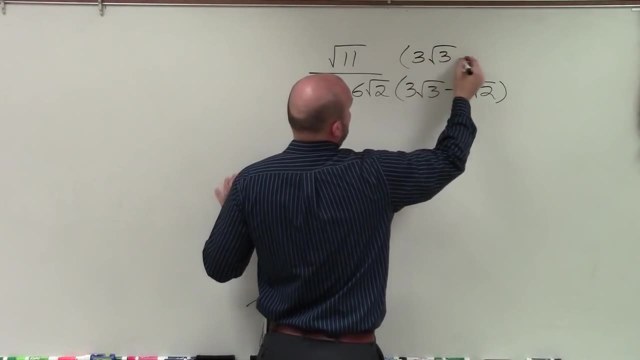 So I have 3 square root of 3 minus 6 square root of 2.. And whenever I multiply in my denominator, I have to make sure I multiply in my numerator. So that's going to be 3 times square root of 3 minus 6 times square root of 2.. Now for our numerator. this isn't so bad, I'm. 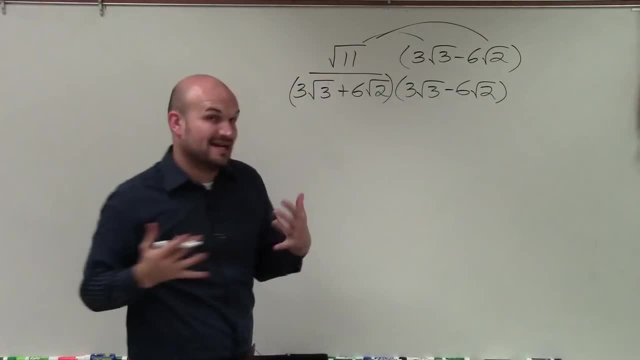 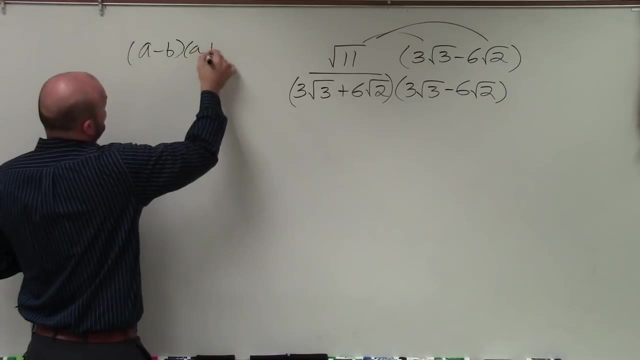 just going to apply distributive property In my denominator. it's not so bad either, because by applying the difference of two squares, all I'm going to have is a minus b times a plus b. I'm just going to have a squared minus b squared. 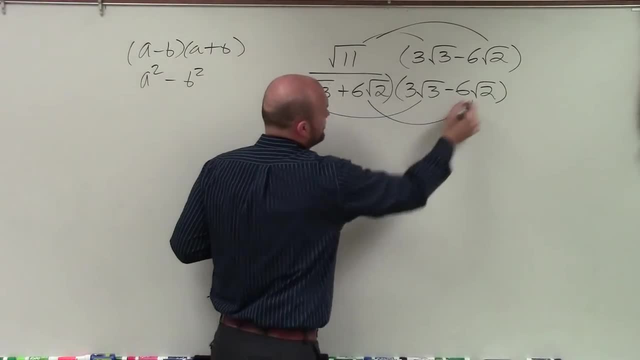 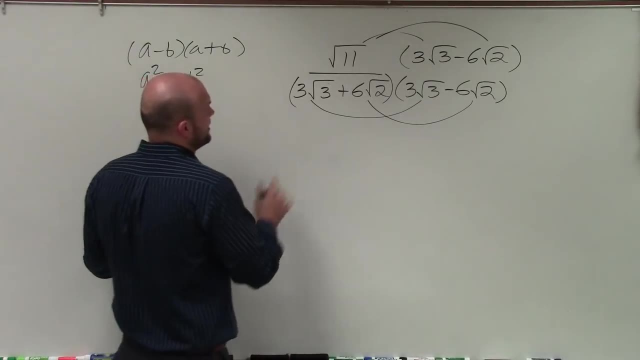 So I'm simply just going to be multiplying my first terms and then multiplying my last terms, because the middle terms are going to cancel each other out or add up to 0, I should say So let's go ahead and do our numerator first here. And the square root of 11 times. 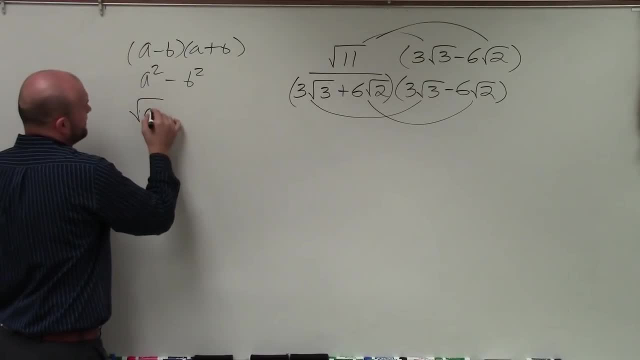 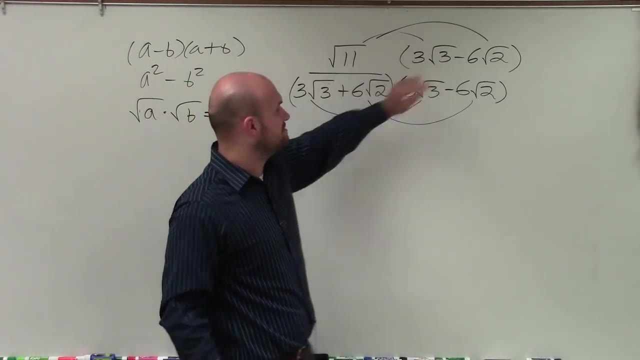 square root of 3.. Remember the product of radicals that states that the square root of a times the square root of b equals the square root of a times b. So therefore I need to multiply 11 times 3.. So I'll have 3 times the square root of 33.. And then when? 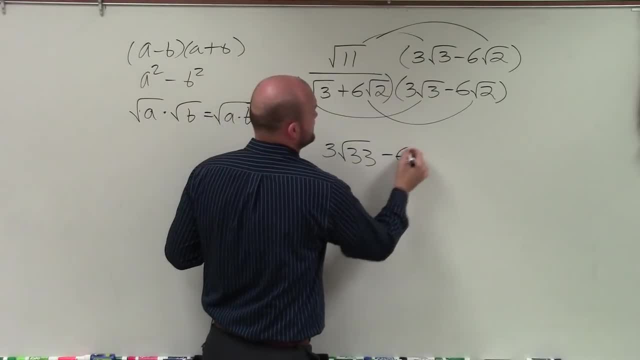 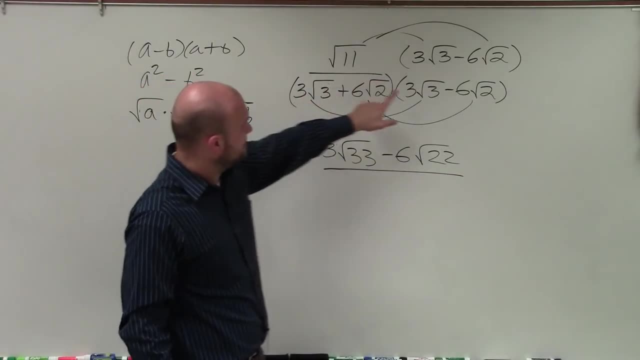 I multiply the square root of 11 times the square root of 2, I get negative 6 times the square root of 22.. That's going to be all over. Now my denominator here I'm going to have 3 times 3, and then the square root of 3 times the square root of 3, which will 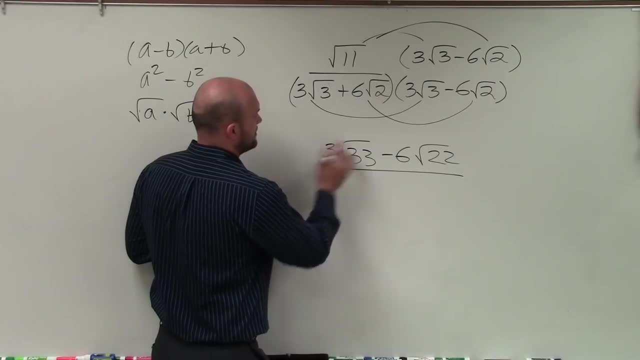 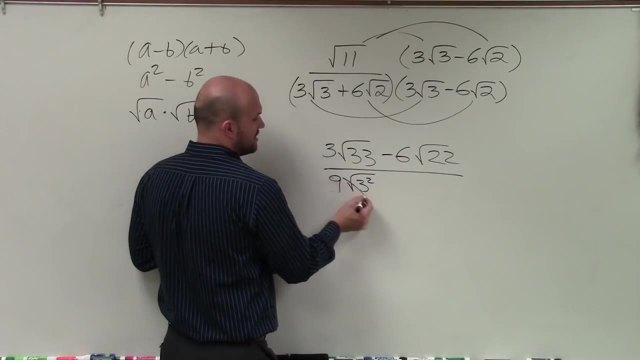 produce 3 times. I'm sorry. 3 times 3 is 9, times the square root of 3 squared. Well, the square root of 3 squared is just going to leave us with 3.. I guess I probably should. 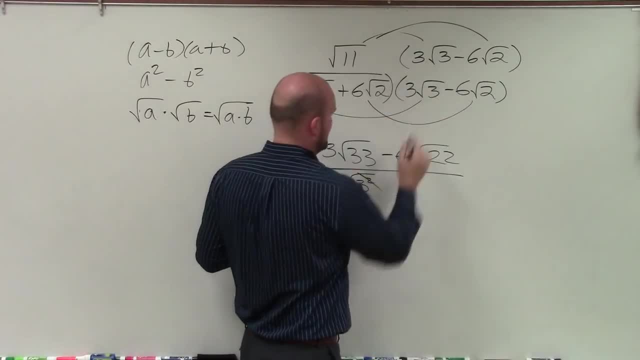 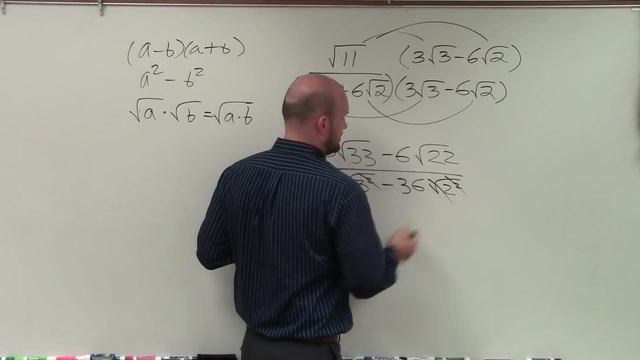 have done the denominator somewhere else, But let's go through it. And 6 times negative 6 is going to be a negative 36.. Square root of 2 times the square root of 2 is going to be the square root of 2 squared, which is just going to leave us with 2.. So I guess, 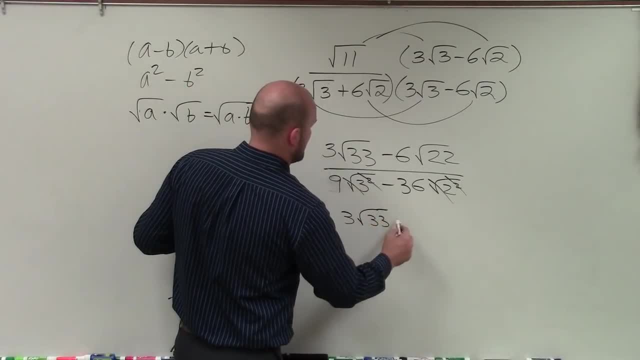 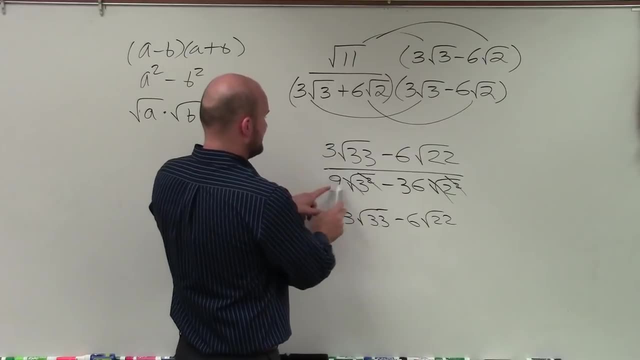 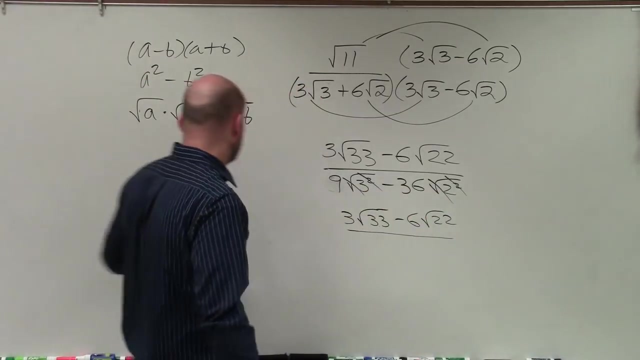 I'll just rewrite it again: 3 square root of 33 minus 6 square root of 22.. And then I can't combine them because they don't have. the radicands are not the same. So I have 9 times 3,, which is 27.. And then I have negative 36 times 2,, which is 9 times 3,, which is 27.. 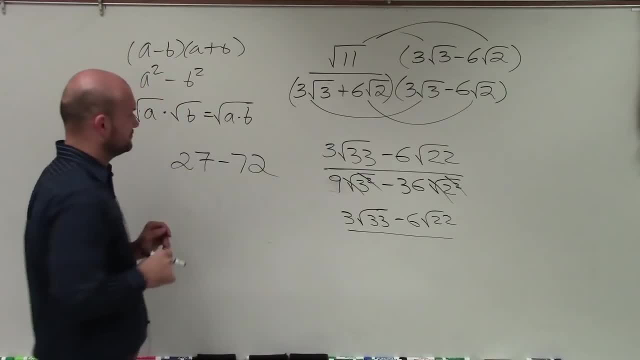 Which is a negative 72.. Right, 36 times 2 is going to be 72.. Now, 27 minus 72 is going to be a negative 42.. No, not negative 42. You're going to add this on. this is going. 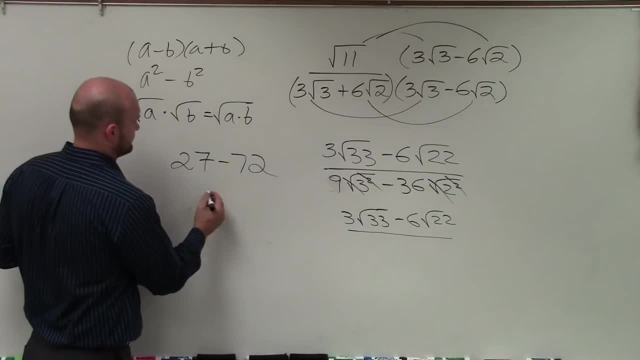 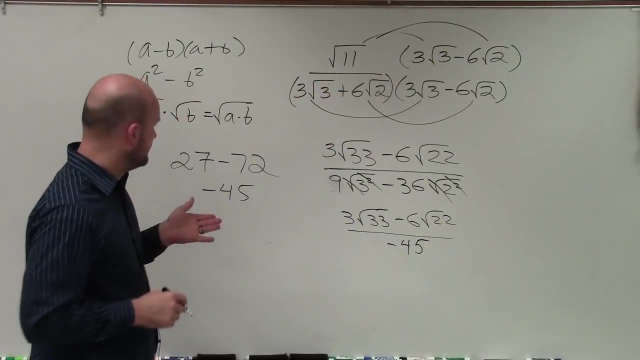 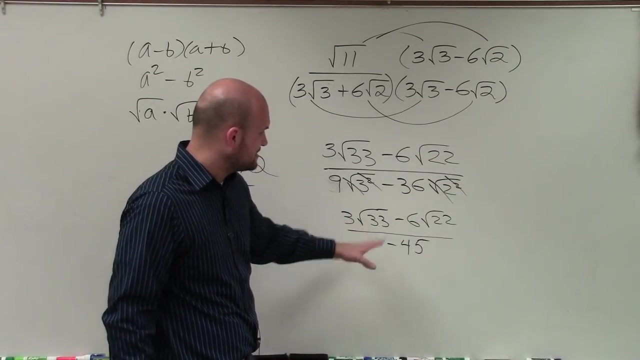 to be a negative 45.. Now, with that, what I can do is I can go ahead and distribute that, I can leave it like this, or I can distribute this to both of them. So I'd have 3 square root of 33 divided. 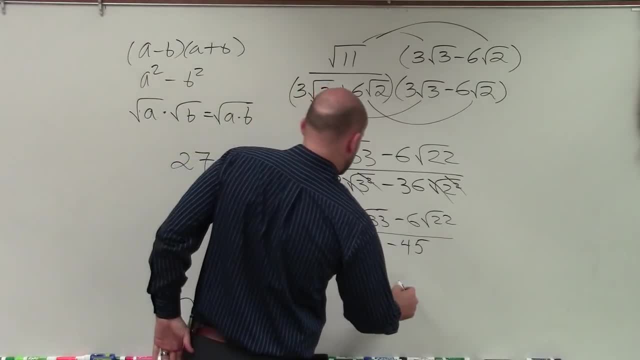 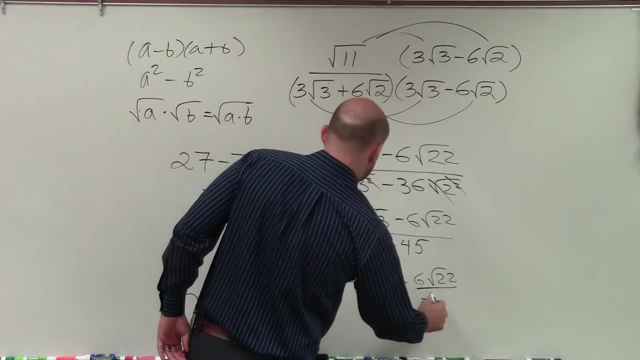 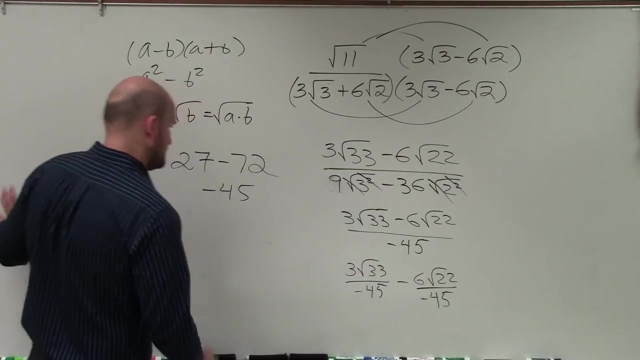 by negative 45 minus 6, square root of 22 divided by negative 45.. And the reason why I do this is because I can simplify 3 over 45 into 1 15th, Or not 1 15th, 15, 30.. Yeah, 1, 15.. So. 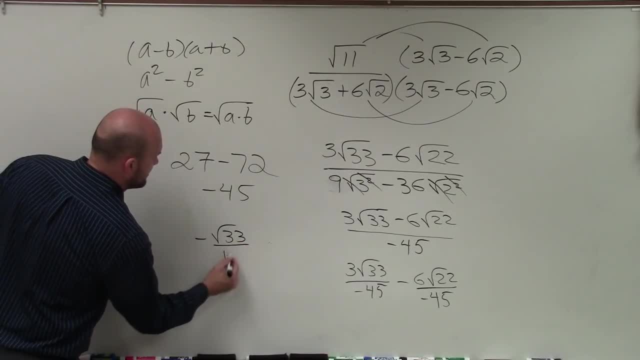 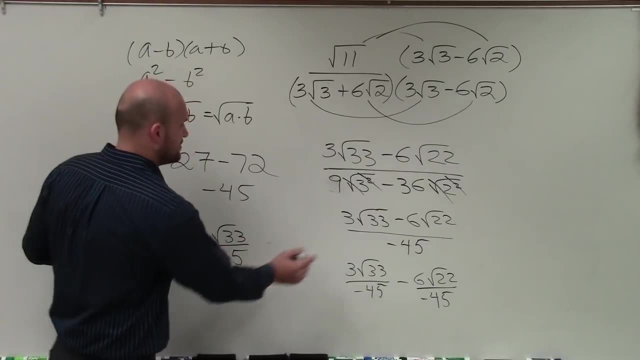 I can rewrite that as a negative square root of 33 divided by 15.. And then I can simplify this: Even though 6 and 45 don't redo, I can divide each of them by 3 again. So negative divided by negative becomes a positive. So therefore, dividing by 3, I would have 2 square. 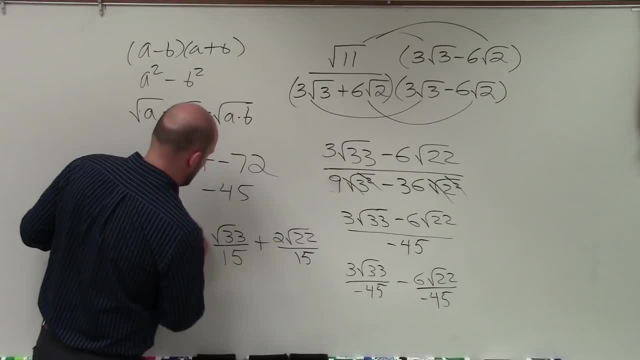 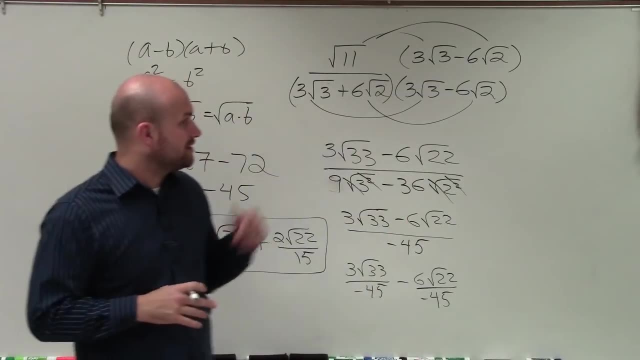 root of 22 divided by 15.. And that's going to be your finalized answer. Or you could also leave it like that as well, kind of depending on what you're looking for in your class. But there you go, ladies and gentlemen. That is how you simplify by rationalizing. the denominator Thanks.